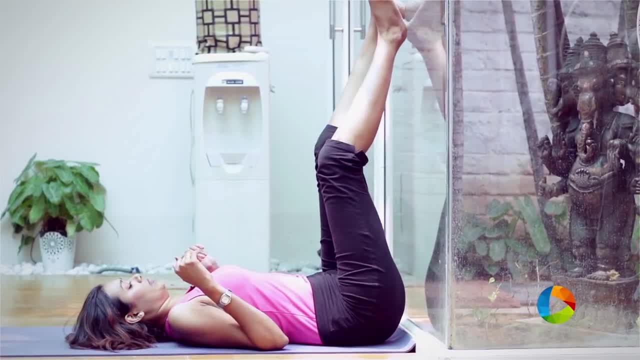 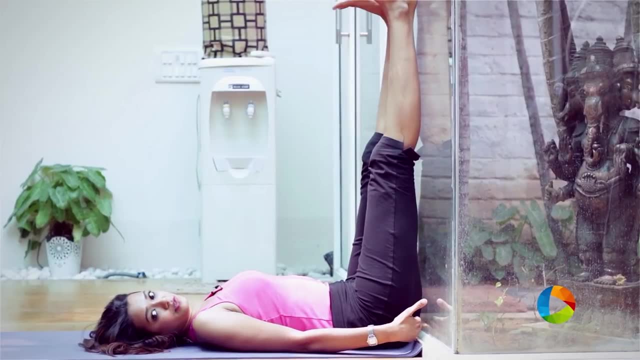 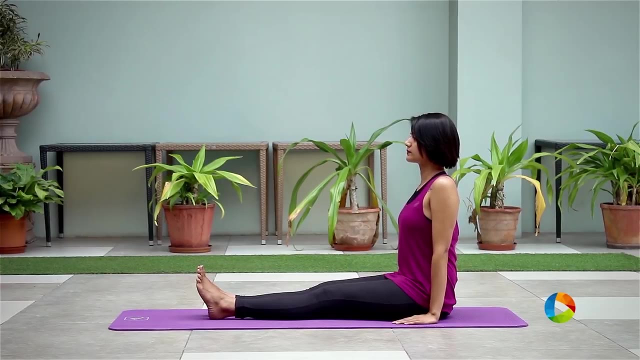 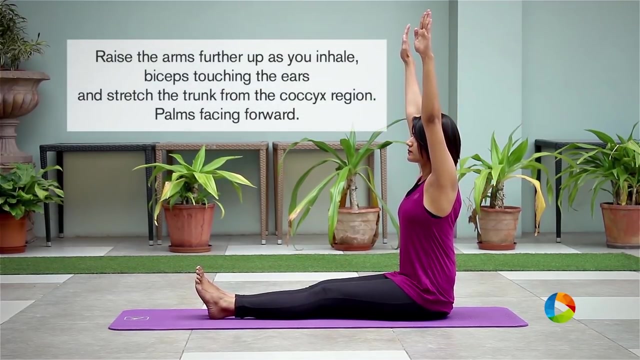 and place both your legs all the way up and still just put yourself closer to your wall. See, my butt is as close as possible- and relax, Relaxing and resting. So the next thing you're going to do will be to look at your weight. 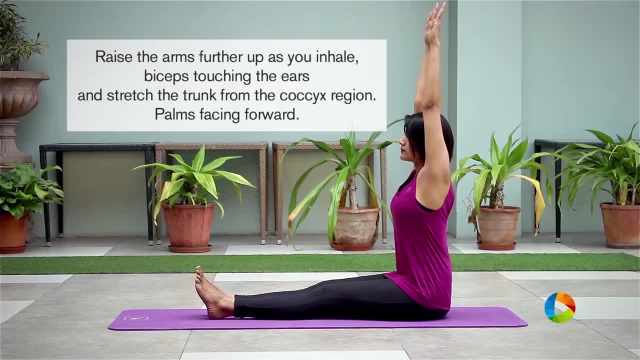 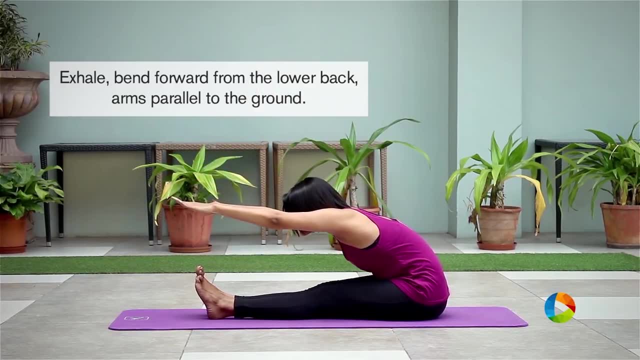 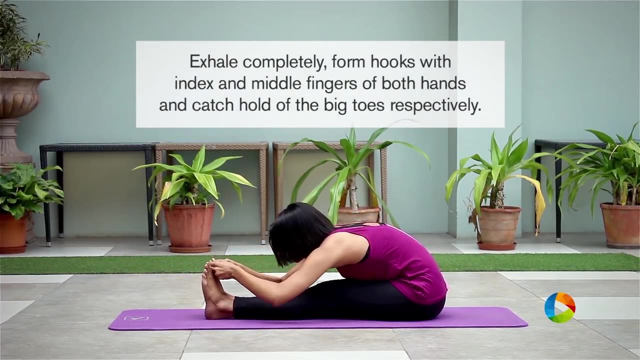 It's a very common thing to do is to look at your weight as if you were looking at your weary weight, because you don't want to feel you're getting heavy. So if you're feeling like this, you're not going to put your weight on your waist, you're. 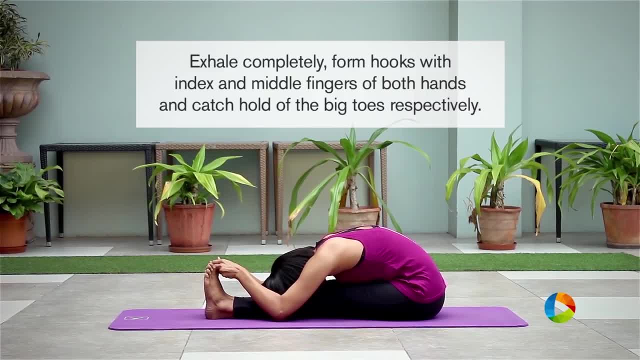 going to pay attention to your weight, So I'm going to put my weight on this side of my body and my back. Just work your legs and feet out. If you're doing this, you're not going to be able to lock yourself up. 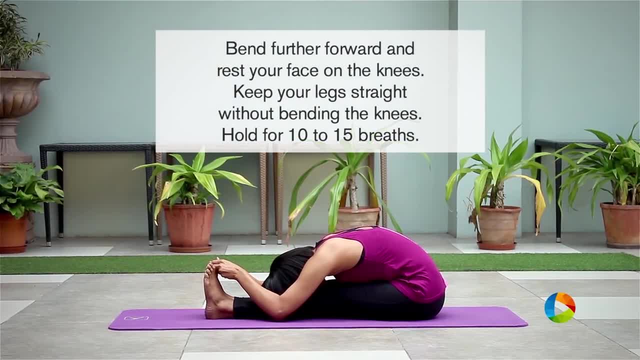 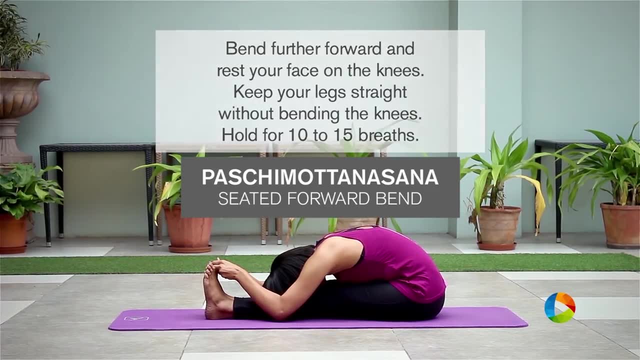 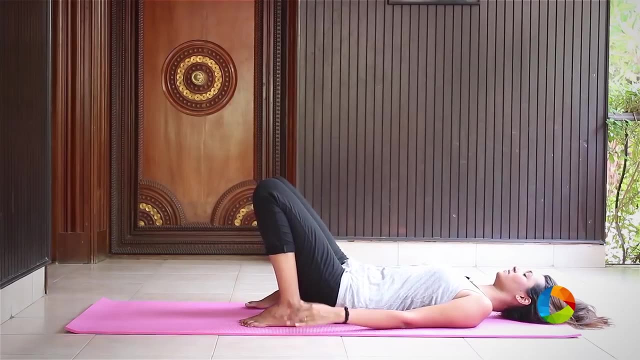 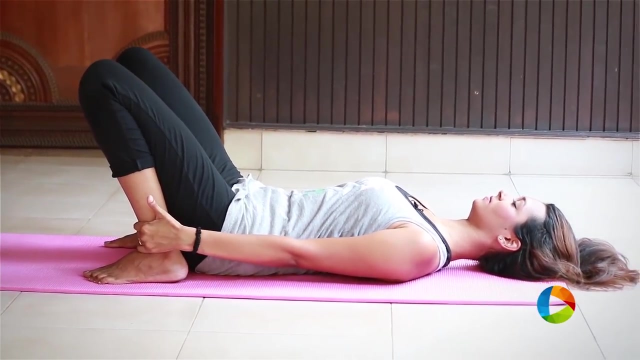 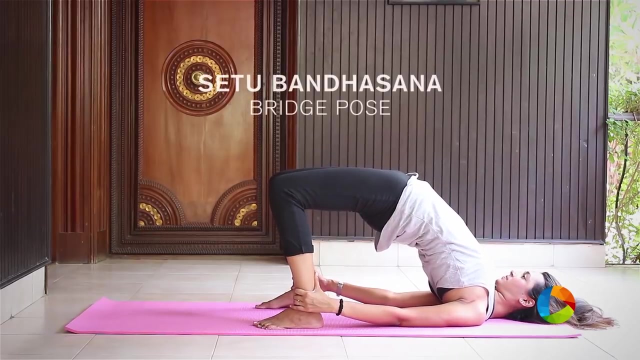 Begin to lie down on your back and place your heels as close as possible to your butt and hold your ankles. make sure your thumb is outside and, when you are ready, slowly inhale and lift your hips all the way up. so try and reach as high as possible, but your breath should be in. 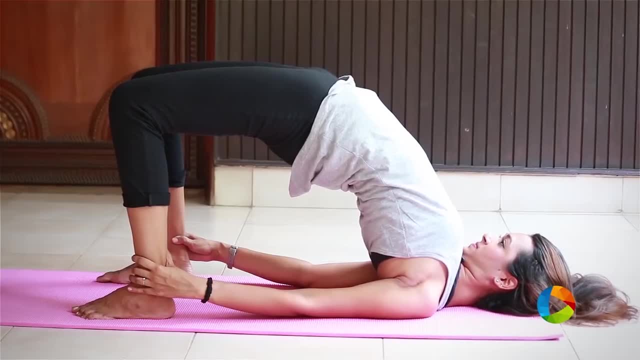 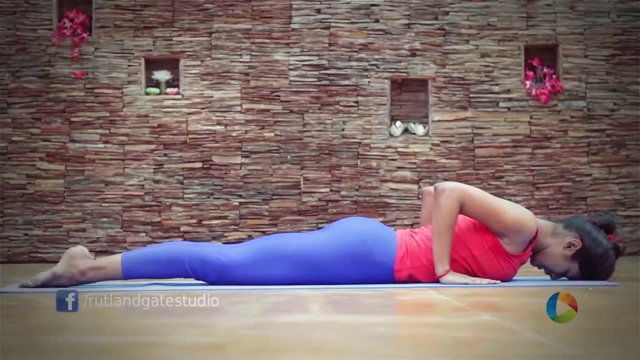 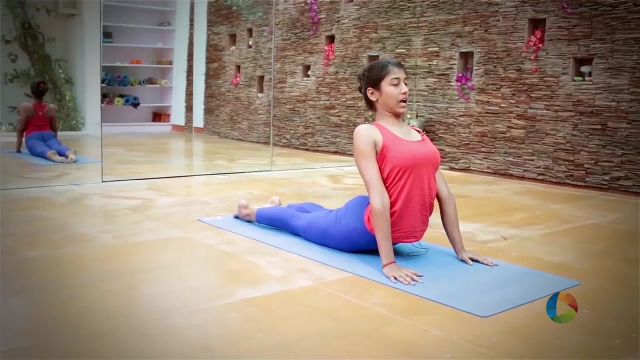 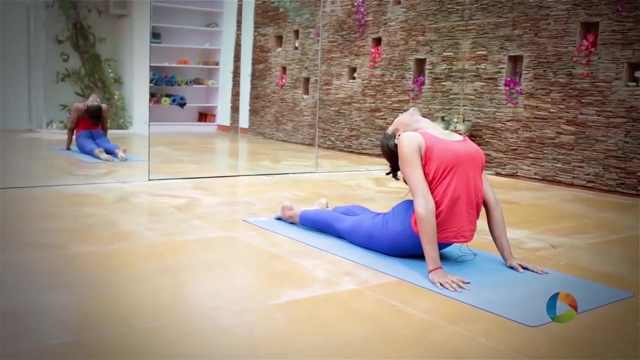 the normal range and stay here for a couple of deep breaths. inhale, lengthen your spine, create a space between your pelvic and your ribcage and then arch back. squeeze your butt, drop your shoulders back and then arch mouth closed. upper jaw and lower jaw in contact with each other. 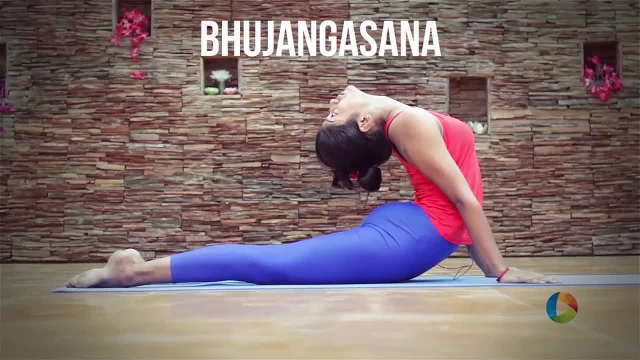 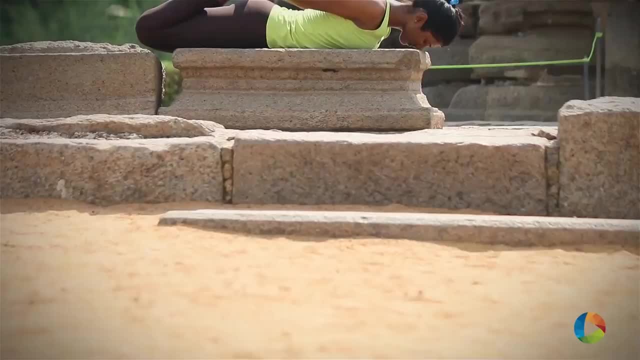 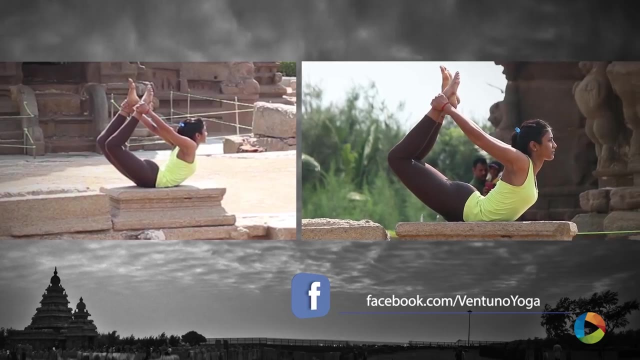 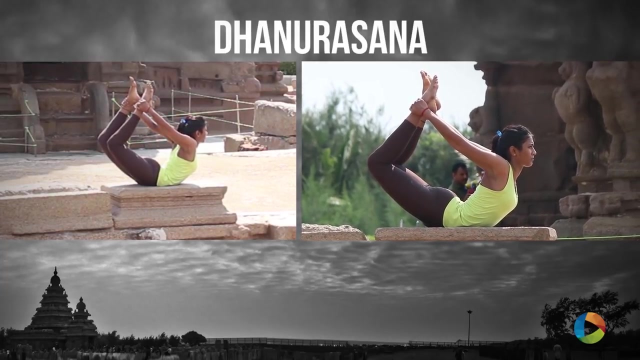 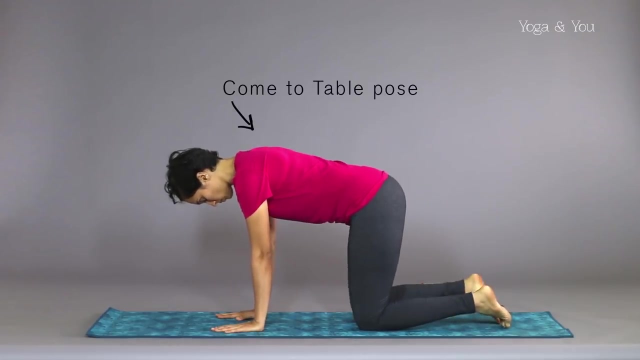 lie down on your stomach. exhale. bend your knees and hold the ankles with your hands wide. inhaling, raise the thighs, head and chest as high as possible. try to maintain the weight of your body on the lower abdomen. join the ankles. look upward and breathe normally sitting on your heels. slowly move on to a table, exhale and lower the.